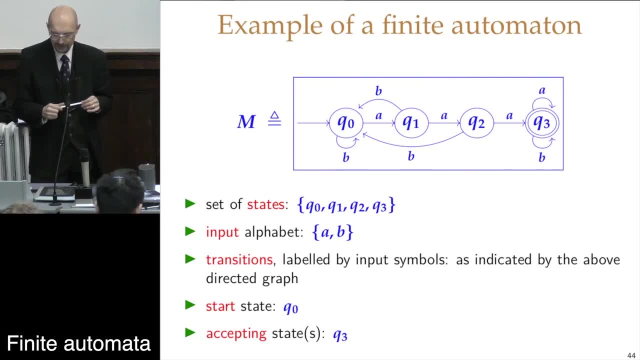 They are the finite state machines of the digital electronics course. We call them automata because it comes from Greek. it sounds more cool, but they are the same thing. Automaton is the singular of automata, which is the plural. They are made of states. 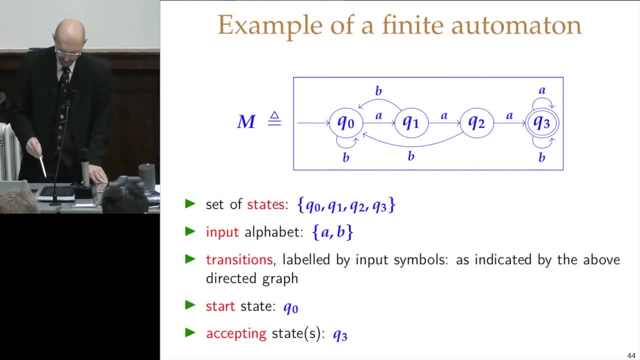 You're familiar with this. States are the blobs. The arrows take you from one state to another state. The arrows are labelled with input symbols And so, if you receive Well, you start in the state that has the incoming arrow. that's unlabelled and doesn't start from another state. 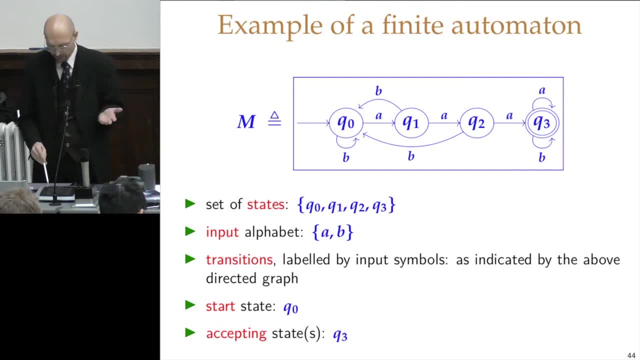 So that's your start state. If you receive a symbol A in this state, you will go where the arrow takes you, which is this one. If you receive a symbol B in this state, you'll go where the arrow takes you, which is this one. 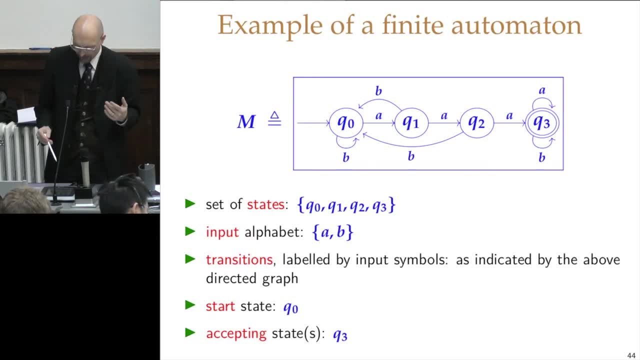 If you receive another B in this state, you go where the arrow takes you, which is this one, And if, at the end of your input string, which in my case was ABB, you end up in a state that has a double border. 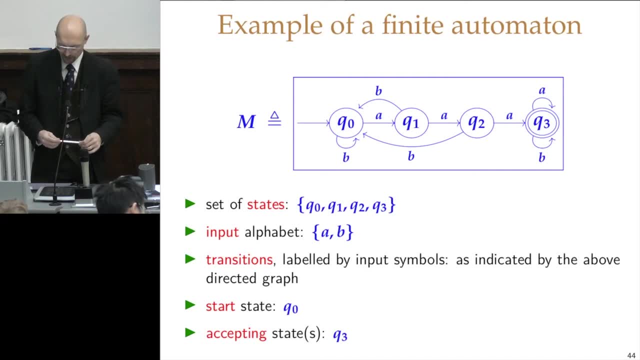 then the string is accepted by this automaton. If you end up with one that has a single border, the string is not accepted. So the string ABB is not accepted by this automaton, Whereas the string AAA is accepted by this automaton. 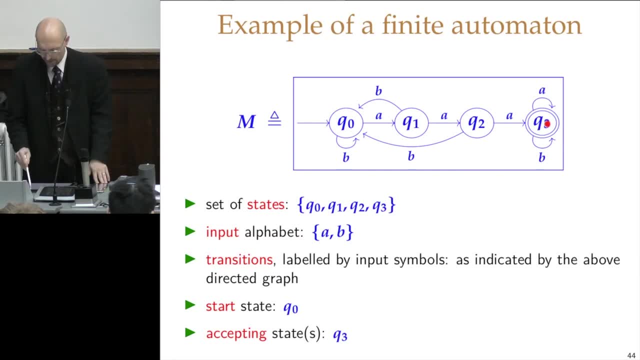 And so is the string AAABBB. You have a set of states. You have an input alphabet Of just the symbols A and B. in this example, The transitions, the arrows are labelled by input symbols. The start state is indicated by this lone incoming arrow. 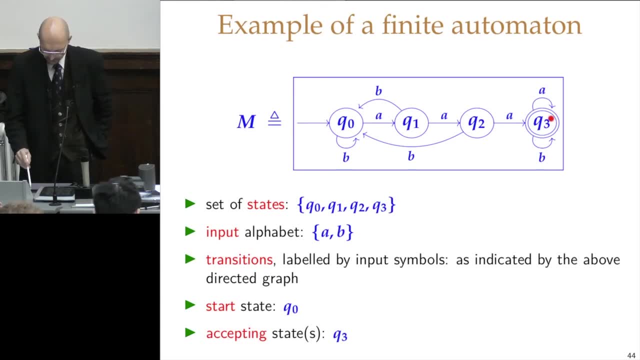 And the accepting states are indicated by this double border. In this example there is just one, But you could have an automaton with more than one state. This one could also be an accepting state. In fact, all of them could be accepting states. 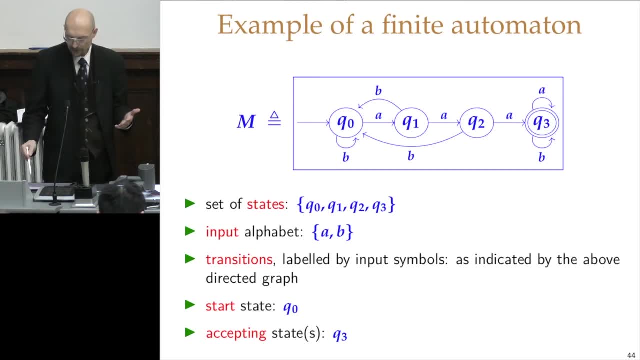 There's no problem with that. You could also have an automaton with no accepting states, And then you wouldn't really need to execute it to know that it will not accept the string. I mean if it doesn't have any accepting states. 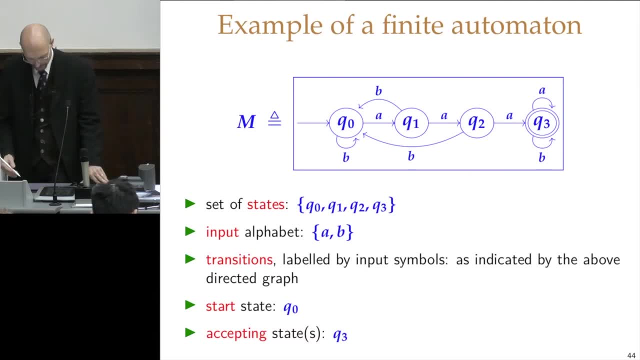 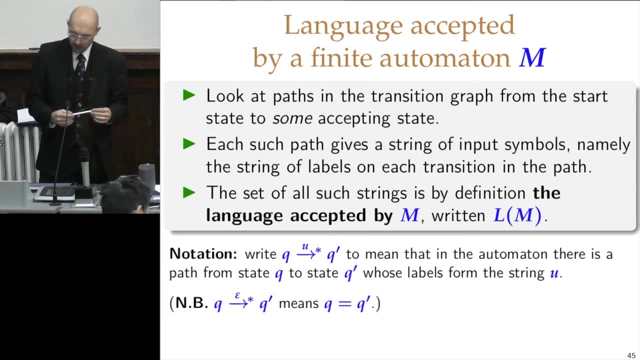 there's no way it's going to accept any string, But it still works like any other automaton And it's still a valid thing for you to define, if you so wish. The language that is accepted by a finite automaton is simply the set of all the strings. 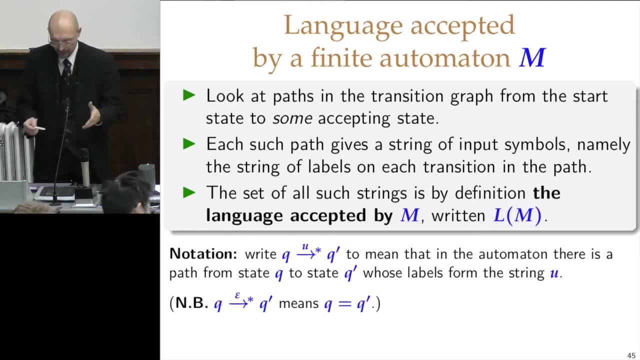 that are obtained in this way. Where is the highlighter? This one. So the important part of this slide is: look at paths. Look at paths in the transition diagram from the start state to some accepting state. We said there could be several. 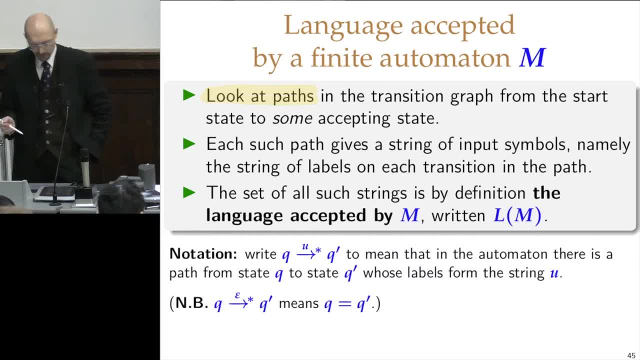 Each such path gives a string of input symbols, namely the strings of labels on each transition in the path. So this is backwards from what you would have done in digital electronics, where you have the machine, you take the input, you feed the input to the machine. 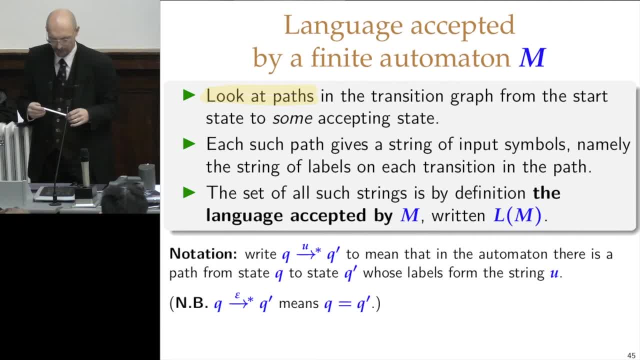 and then you see if it lights up with an accepting state. Here you're doing the reverse. You're taking the machine, you're looking at all the paths and every time you find the path that finishes in an accepting state, having start in the start state. 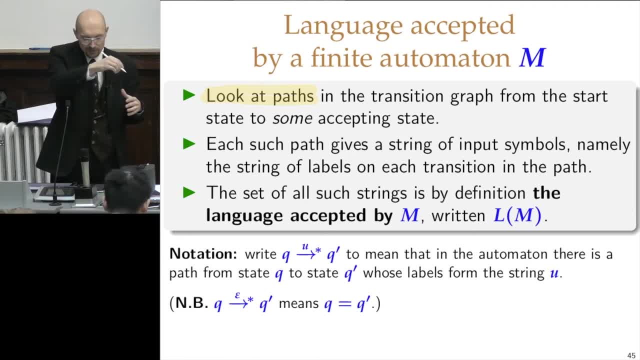 then you say: the string of symbols that I encountered along this path is a string that this machine has, This automaton accepts. I say: go this reverse way. Why are the two things not quite the same? This is notation, so let's just get the notation out of the way. 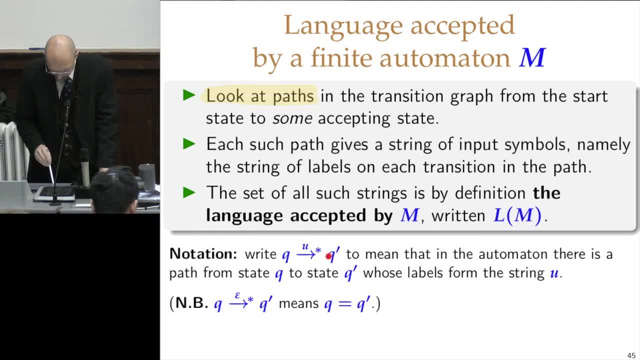 Previously, we had just one arrow between one state and another state and a symbol on top to say: with this symbol, I go from this state to this other state. Now, this is not a symbol. It's a meta symbol representing a string. 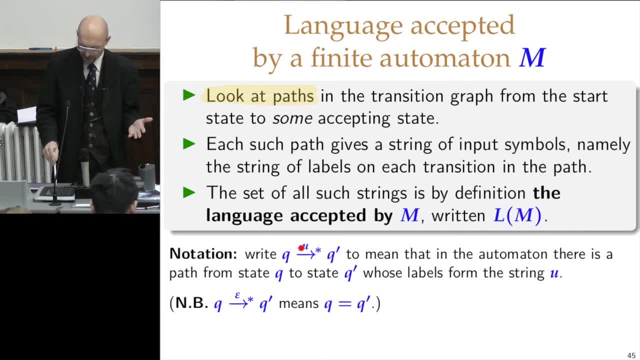 and so I put a star next to the arrow saying if I get a string, then there's a sequence of zero or more arrows that take me from this state to this state. Or, with the alternative view I've given you, there exists a path taking me from this state to this state. 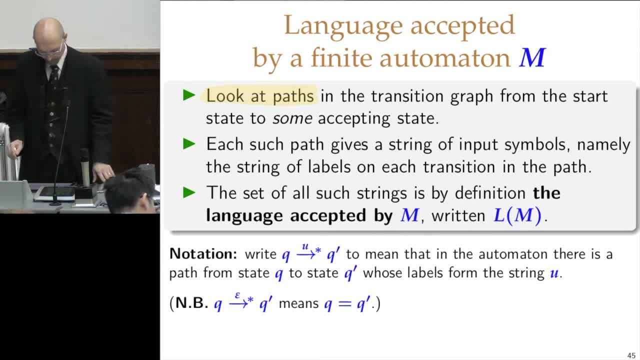 where the labels on all the transitions form the string here. So if you put epsilon at the empty string over here, then it means there is a path made of zero arrows. that takes me from q to q prime, which means q prime is the same as q. 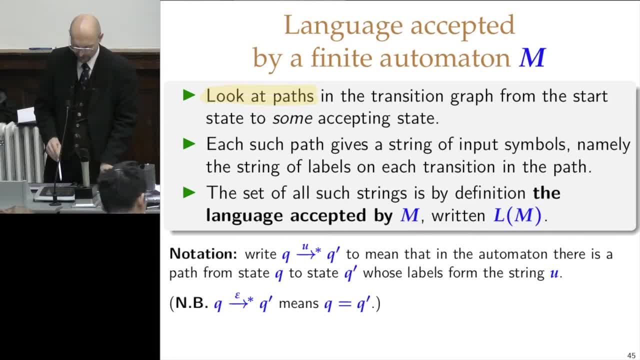 There's a path of length. zero means I end where I began. But I was saying: why are the two things looking at it, from the string to the accepting state or from the path to the string, why are they not quite the same? 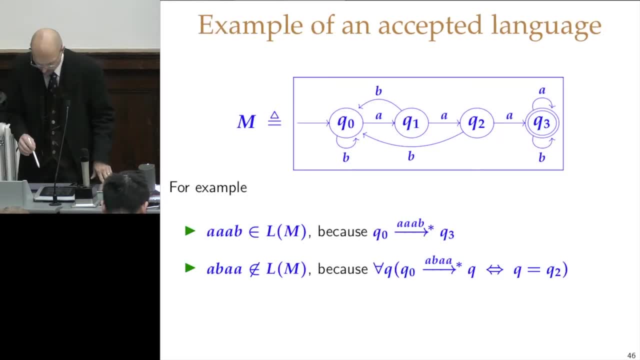 And we will see that in just a moment. Here's another example. Always worth playing a bit with examples before doing all the theory. Same for when you write your own answer to an exam question. Just if you have a grand theory, just try it on a small thing and see if it works. 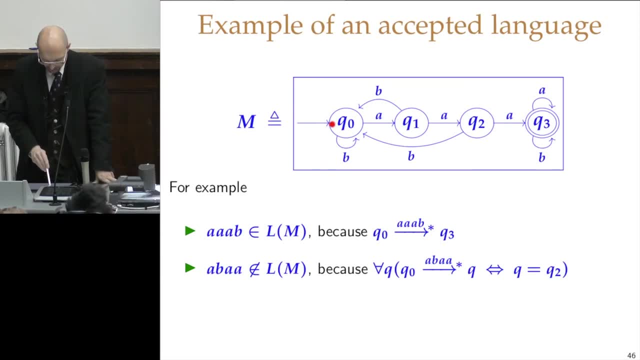 This string: a, a, a, b. if I start in this q zero state, a takes me to q one, a takes me to q one, a takes me to q three and b takes me again to q three, which is an accepting state. 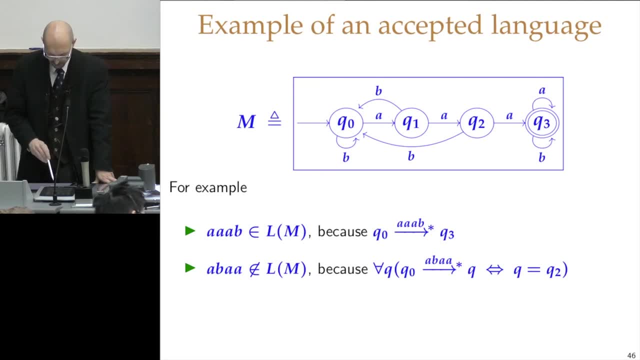 and therefore this string belongs in the set l m of the language recognized by this machine, m because there exists a path from q zero to q three, which is an accepting state whose transitions are labeled a, a, a, b. Now, a, b, a, a does not belong. 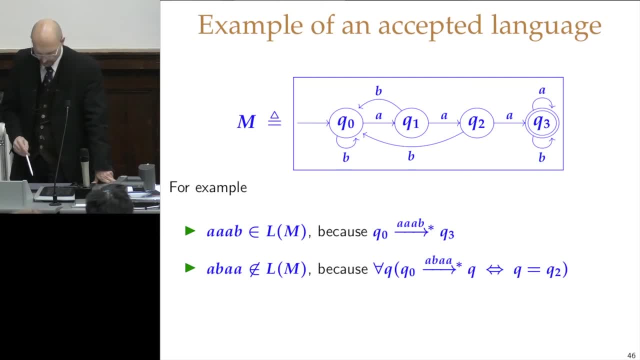 in the language of this machine m, because for any state q, such that I go from q zero to q with the string a, b, a, a, then it so happens that that state is q two. It's a strange way of saying it, but it means. 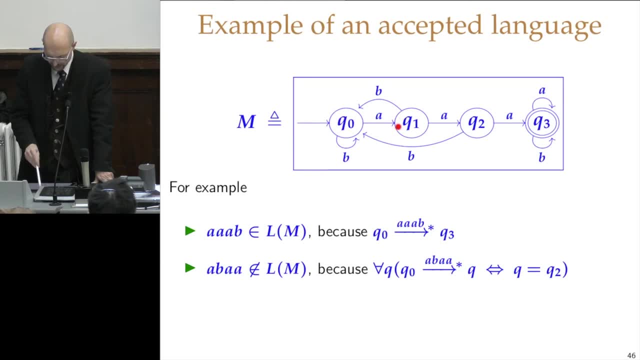 okay, well, I'm here I go. a, b, a, a. the only place I could end up in is q two For all q's that take me somewhere from q zero with this string. it so happens that all these states are q two. 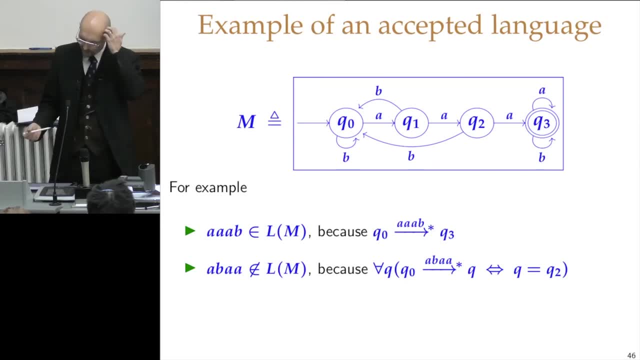 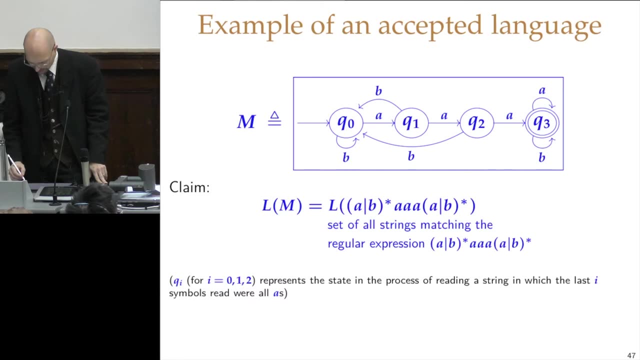 That is the only state that does that. This seems very contrived, but we are saying that for something that will become clear in two slides, So let me go back here, but if you wait until that other slide, we will see why that made sense. 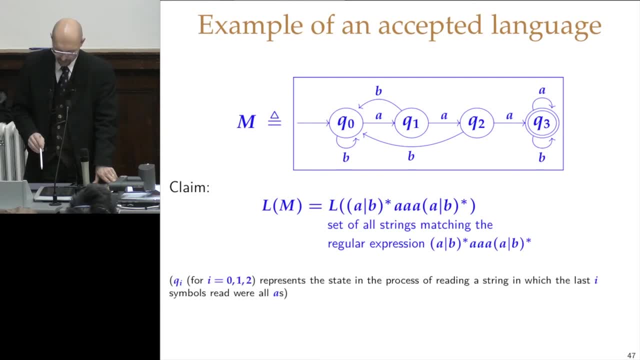 So this here is an attempt at interpreting what the language recognized by this is, And I'm giving you the insight that the language of this machine is the language that would be recognized by this regular expression of having an a or a, b as many times as you like. 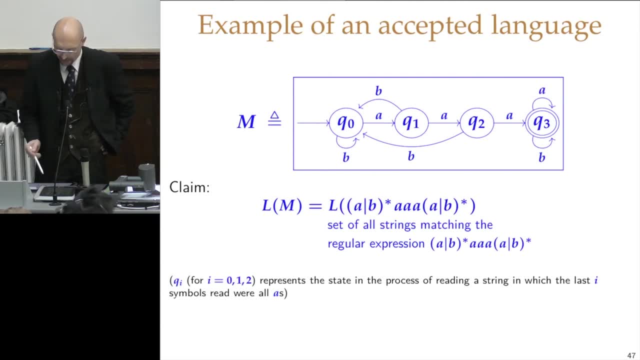 then three a's, and then an a or a b as many times as you like. So you can have an a or a b as many times as you like. That's not quite so obvious, this part. I mean having three a's. 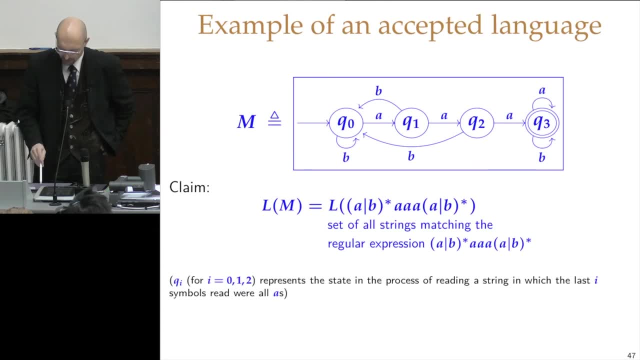 and then an a or a b as many times as you like. that part is pretty obvious. This part you need to think about a little more, And it would be useful if you actually did think about it on your own. But it is true that, if I have 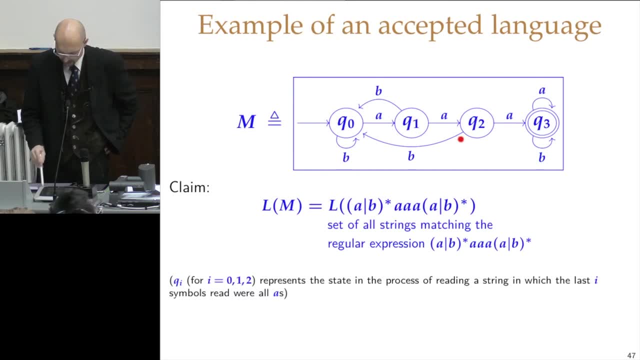 I can have an a and a b, or a a and a b, and what happens is that I can have b's. I can have more b's- a, b, b, b, b, b, b, b, Whenever I try to make a string of things in here. 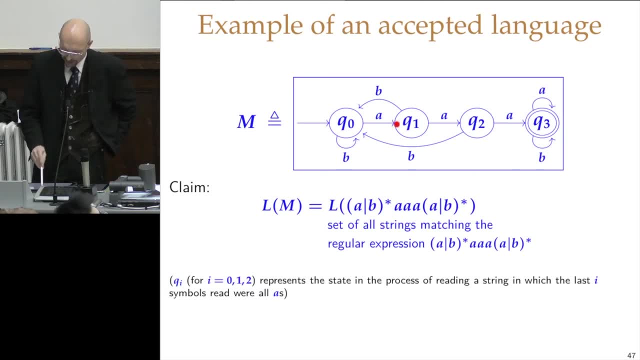 I'm actually trying to go through these three, But so long as I haven't reached the third one, then I'm sent back to the start, So you can see these states as counting. how many consecutive a's have I seen Here? I've seen zero consecutive a's. 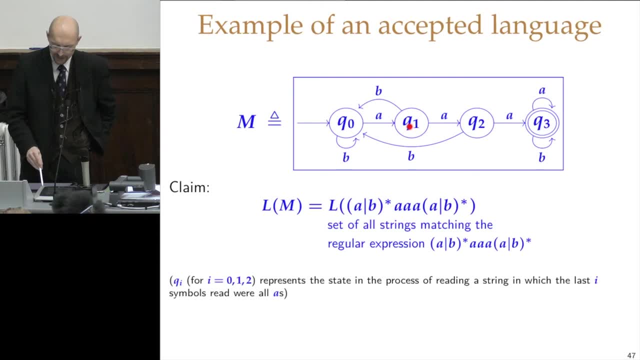 Here I've seen one consecutive a, and if I get another a, I've seen two consecutive a's, Because if I get a b, then I have not seen one consecutive a anymore, because I have to restart from zero. And then here I've seen two consecutive a's. 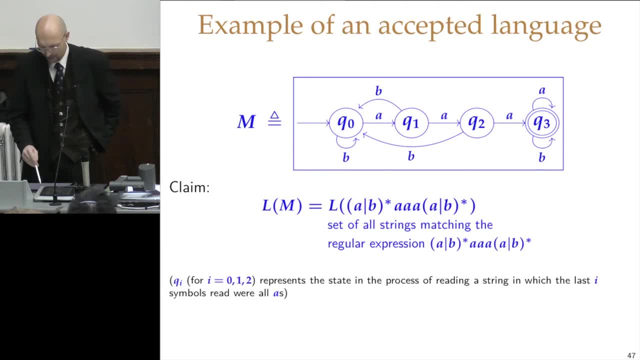 If I see another a, then that's three consecutive a's, which is already an accepting state, because I can already stop here, But if not, I go back to zero. I have to start again. So that's how this is obtained. So I'm always making attempts at this. 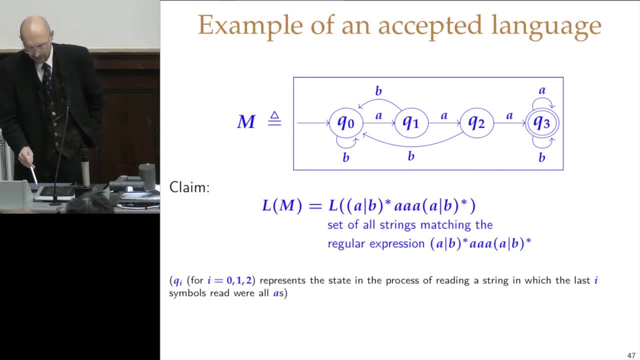 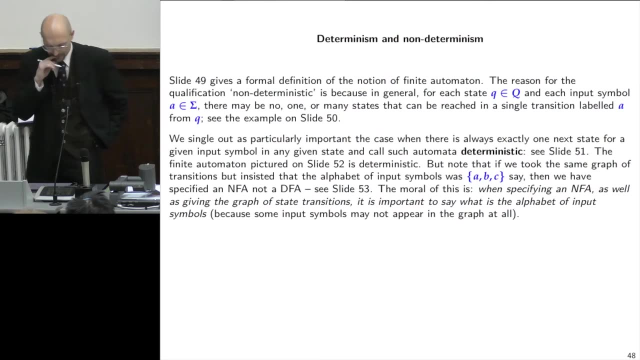 and if, if I get a, b in between, then I say oh sorry, that was not here. actually I was in here. So the thing we wanted to say for a while was that the computation that given the state I'm in and the symbol I receive from the input, 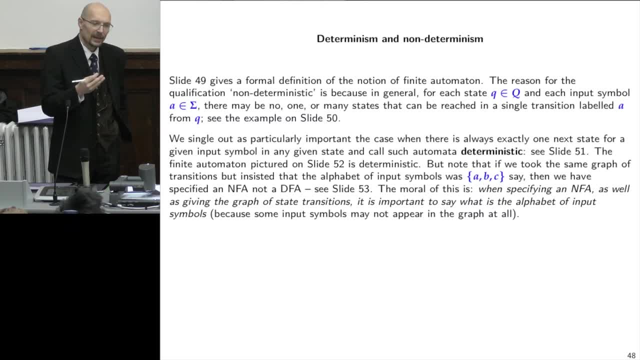 sends me to another state might, in the general case, not send me to one other state. It might send me to one of several possible states, including none. If that is so, then this is a non-deterministic, finite automaton. If, instead, it sends me to exactly one, 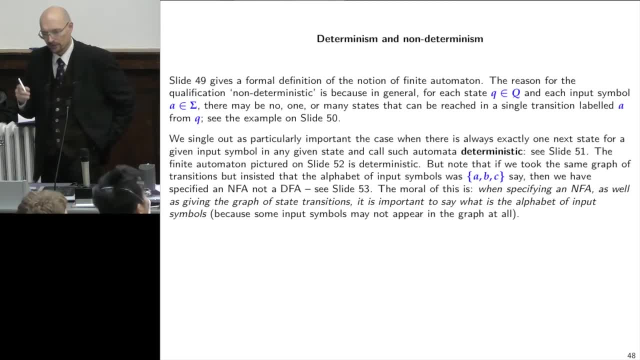 for every possible combination of state and input symbol, then I call it a deterministic finite automaton. And the ones you've seen in the discrete in the digital electronics course were obviously deterministic finite automaton. But now that we are more in the realm of theoretical computer science, 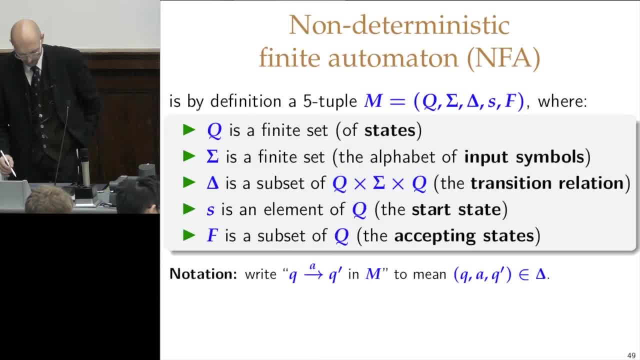 we are happy to explore the non-deterministic version. So the non-deterministic version has a set of state set of states, a set of symbols for the input alphabet and then a relation capital, delta, which is, in the most general form, just a subset of. 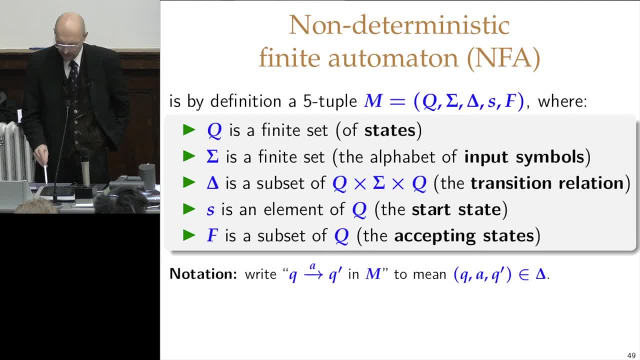 the Cartesian product of the starting state, the input symbol and the ending state for that transition. So if I'm in the starting state and I receive that input symbol, then this is a relation, a generic relation. it's not a function from this to this. 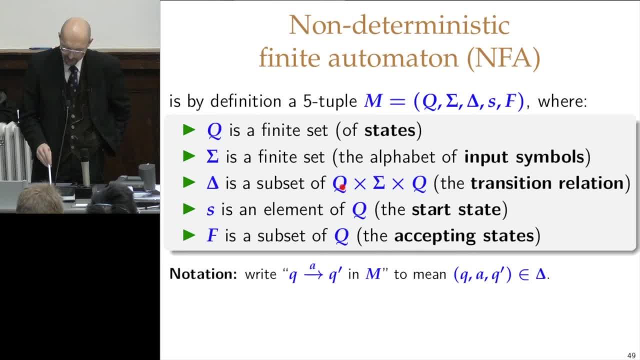 So I can have many tuples where I have the same starting state q0, the same input symbol, a, and many. I can have a tuple that says qa, sorry qa, q0 a, q0, it could say q0 a, q7,, q0 a. 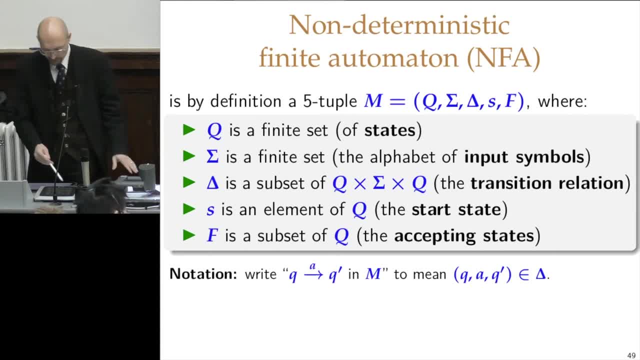 q19 and they're all valid tuples of this relation. So when I'm in q0 and I get a, I might go into any of the things for which there is a tuple. That's the non-deterministic part, including none. 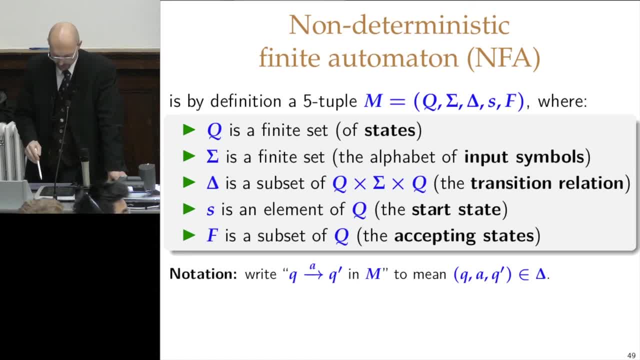 This, there might be no tuple for a certain combination of input symbol and input symbol and starting state. S is a specific state designated as the starting state and F capital. F is a subset of the states that are designated as accepting. The subset can have as many states as you like, including all of them. 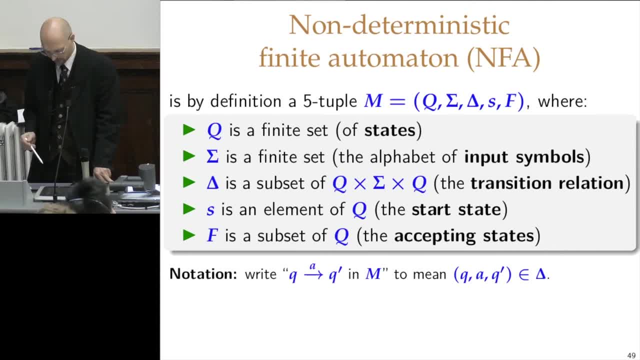 including none of them, including exactly one, including a number different from one or zero, or all of them. And so this notation. we've already seen that there is a transition from q to q prime with input symbol. a simply means that the tuple q, q prime and a. 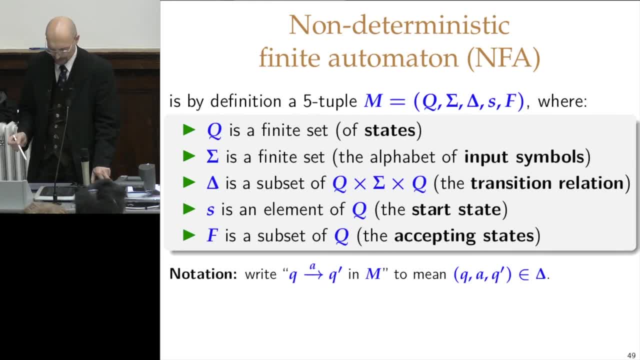 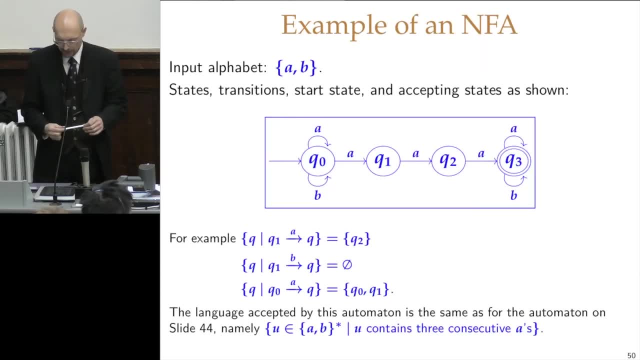 is in the relation delta that defines the allowed transitions of this automata. So here we have an example of a non-deterministic finite automaton which recognizes the same language as the previous one. And I'm not proving that to you, I'm just telling you. 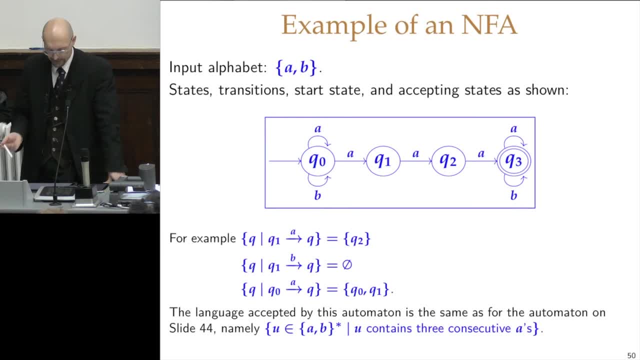 It's again all the strings that start with anything, finish with anything and have at least three a's, three consecutive a's, somewhere. So this one, you can see, starts with anything, can have a's and b's, and you stay here for as long as you play with the. 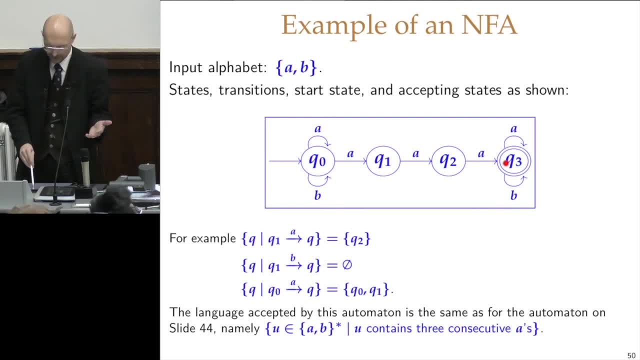 strings Start with anything, Then when you decide to have your three a's, you have your three a's and then you can continue with having anything in here. But notice, the thing that makes this an NFA is that from q0 you can go with an input symbol of a. 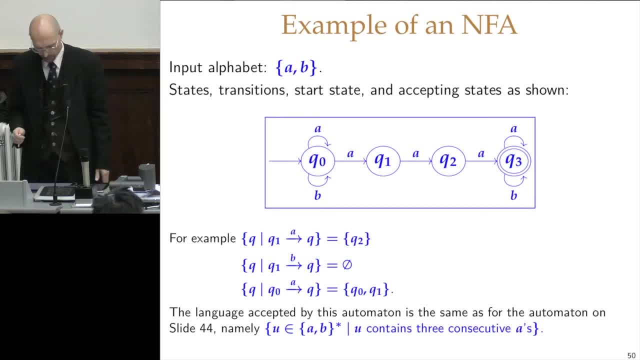 you can go to q0, you can also go to q1. It's up to you to do one or the other, and both are valid ways of using this machine. There is a path in in this machine from q0 to q0. there is a path from q0 to q1. 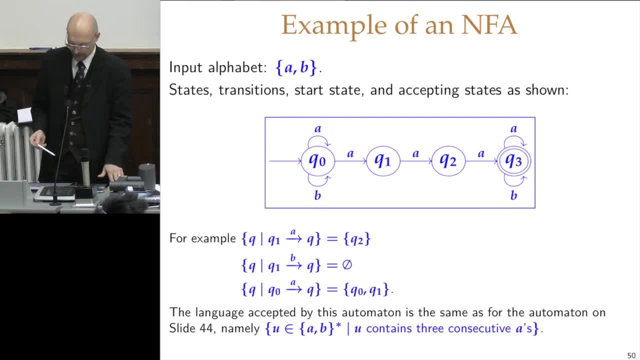 with the string a and so on. So both of these, all the ones, all the paths that end in q3, are accepting the language This stuff. turn here and go here, or just don't waste any time here, just go straight here or go here. 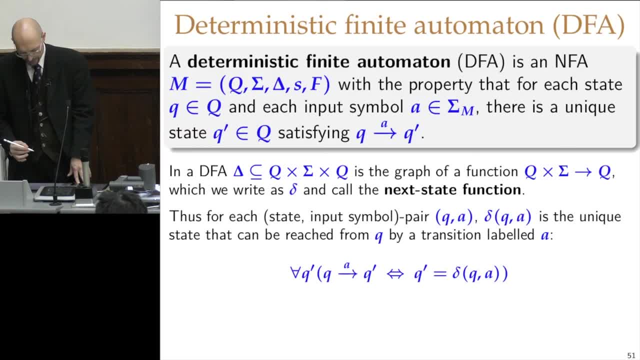 do plenty of that and so on. They're all fine. The deterministic finite automaton instead is one where this relation delta has a unique value for the, for the third element of the tuple, once you have chosen the first and the second. So if you fix, 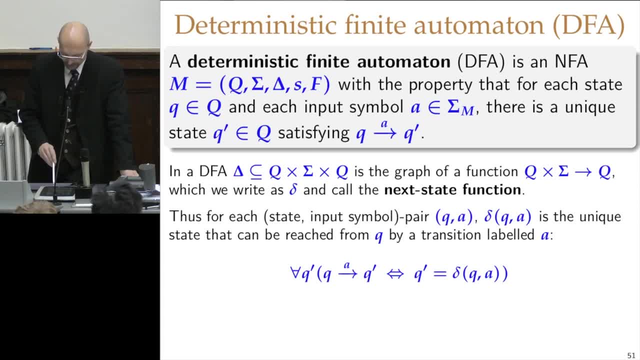 the state and input symbol, then the destination state is unique in the deterministic finite automaton And so we indicate this relation, which is now a function from a- q, because it's a function we indicated with the lower case delta function of q and a And it has a. 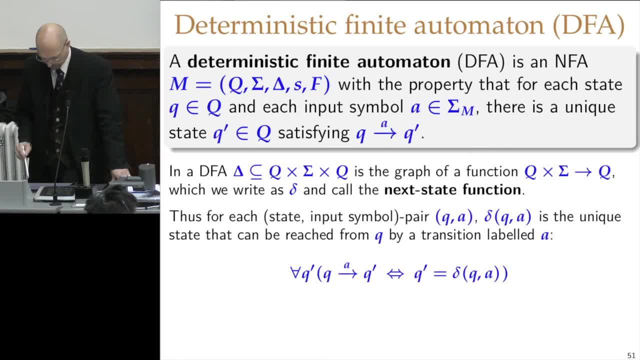 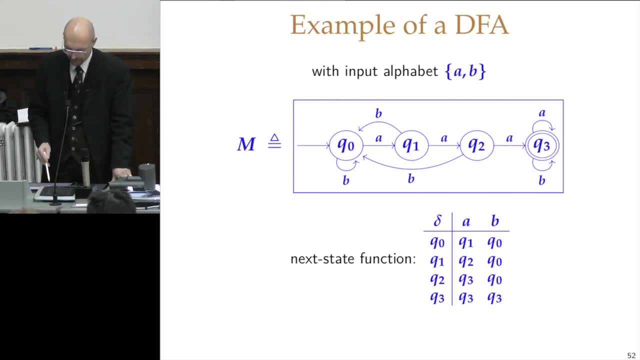 unique result, which is a member of q, So the one that we had originally was a DFA, so we bring it back again. and here's the DFA for recognizing the strings that have three consecutive a's, and you can tabulate the next state function as you have done in digital. 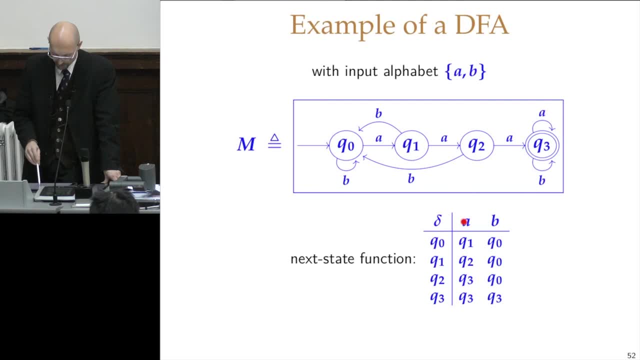 electronics by saying: if I am in this state and I receive this input symbol, then I go to this state. if I'm in this state and I receive this input symbol, I go to this state, and so on, And then you can use this, taking a string of: 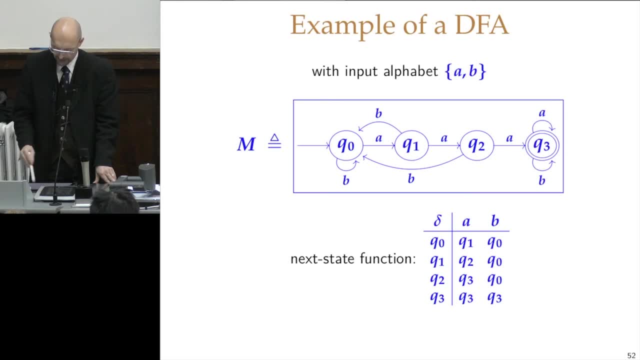 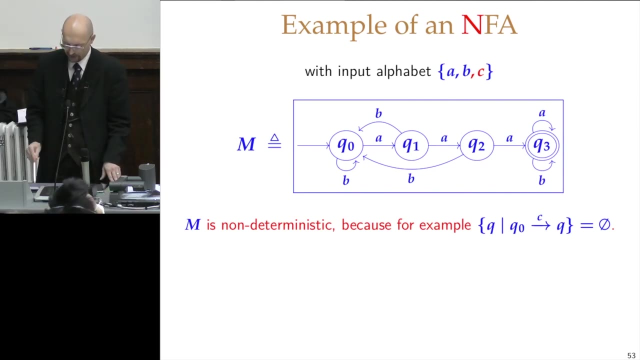 input symbols, navigating through this by one look up at a time and seeing whether you end up in an accepting state or not. This is perhaps surprising. it's the same diagram as before. it's exactly the same, but it is now a non deterministic, finite automaton. 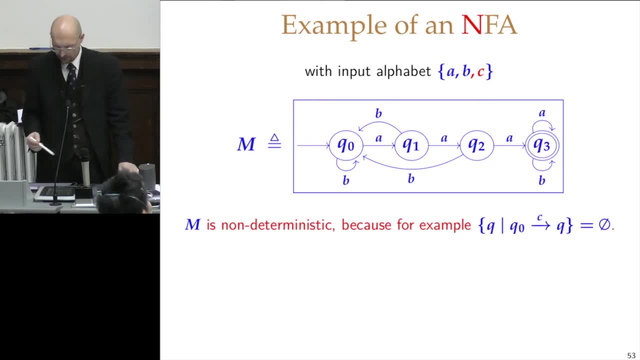 for the small, almost imperceptible change I made of redefining the input alphabet to also include the input symbol c. The diagram has not changed at all, but the fact that I now also have the input symbol c means that there is no longer a function that assigns. 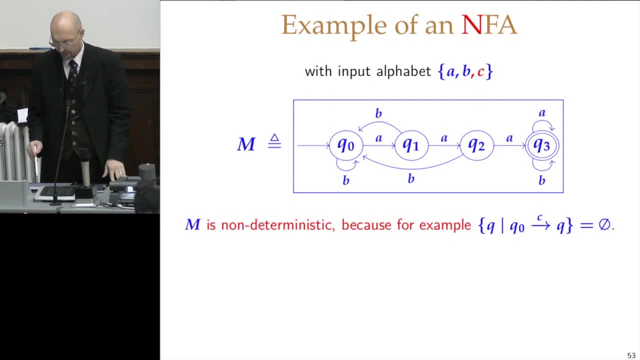 a uniquely determined next state to every possible combination of state and input symbol, because if I am in q1 and I receive the symbol c, this doesn't say what happens. in fact, nothing happens, and so this is what makes this non deterministic, and so this highlights the fact. 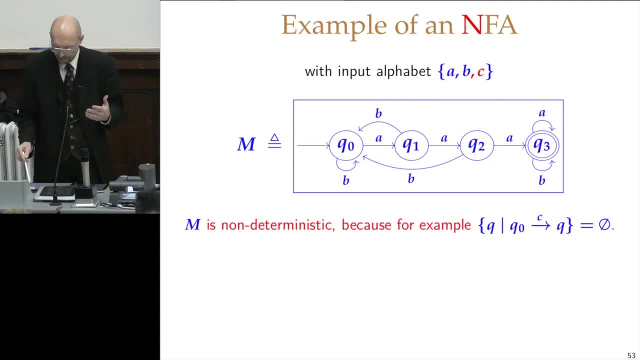 that you cannot speak of the machine just by giving the diagram without having also specified clearly what the input alphabet is, and you cannot gratuitously infer the input alphabet from this just by reading things that are on the labels, because there's nothing to say that there aren't other symbols. 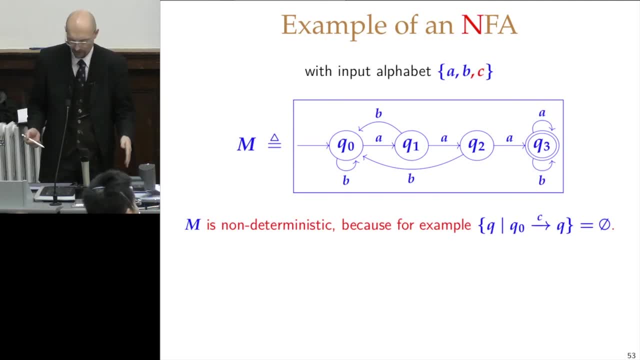 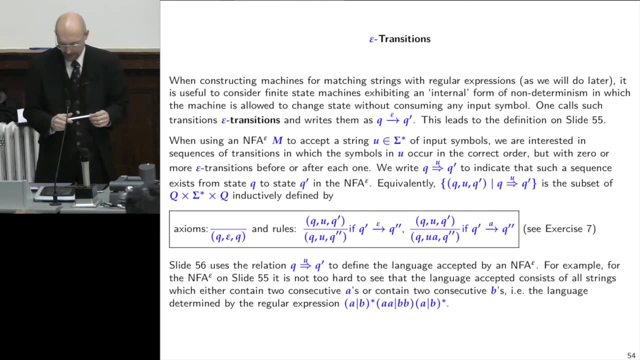 in the input alphabet that never appear on any label, just as in this case, and that would make the difference between being a DFA and an NFA. What I'm introducing here is some non determinism inside the machine by having ways of moving from one state to another. 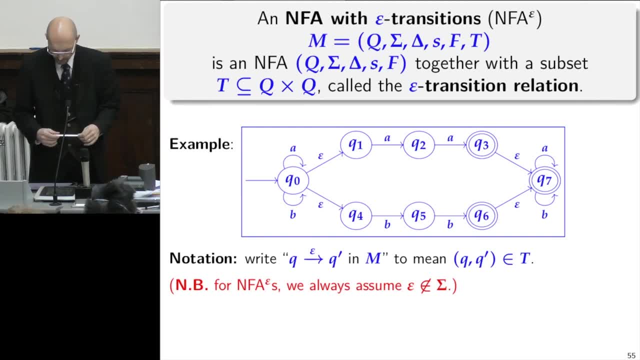 even without receiving an input symbol, and I'm free to do that or not. so I'm in here, I'm in this state, q0, and if I receive an a, I go to q0. but I don't need to receive anything to be free to go to q1. 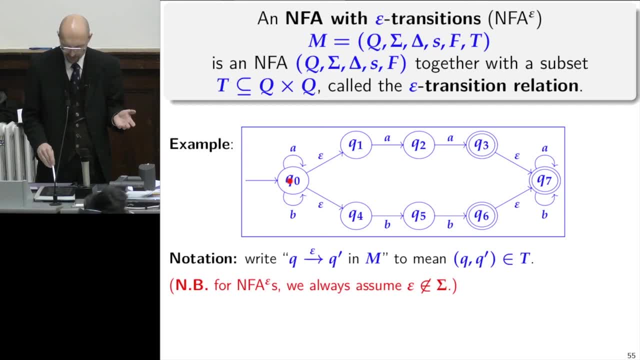 so I can say that after the string a I'm in q0, but after the string a I might be in q1, because I've done this transition and then I've done this other one which I can do for free. so when you have an epsilon transition, 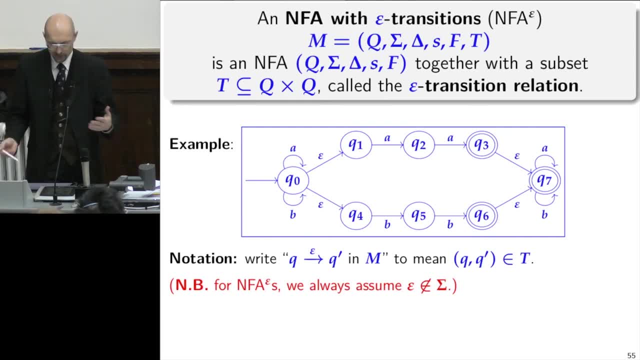 you can take it or not take it, but you don't have to consume any input symbols to do so. and so, if you take the other view, look at paths in this automaton from the start to any accepting state. there's three in this case, so I look, for example, at the path that goes. 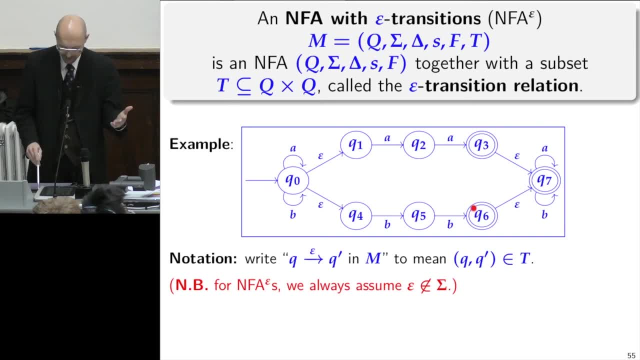 ab epsilon bb into an accepting state. so it means the string ab epsilon bb. if I drop the epsilons, ab bb is a string that's accepted by this automaton. so take all the paths. take any path from the start state to any accepting state. read out: 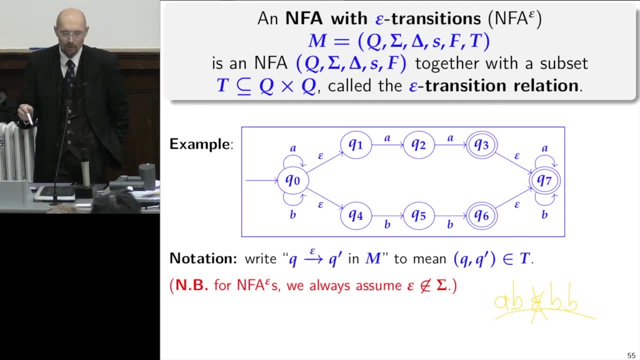 the labels of the transitions that you traverse. drop all the epsilons and that's an accepted string in your language. just to keep our sanity we keep separating the meta symbols from the symbols because otherwise things become too messy in the regular expressions that you use on your computer. 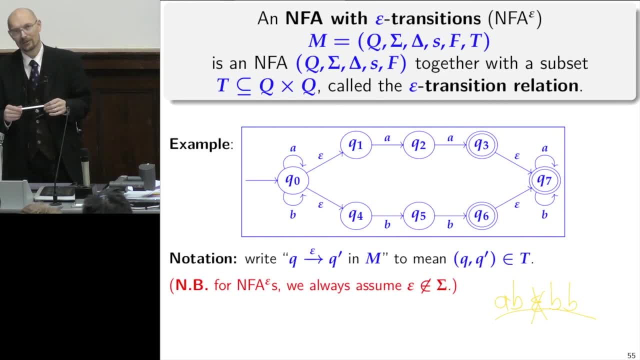 you have this complete garbage of backslashes everywhere, because the same meta symbols that describe the extra stuff of the regular expression have to come from the same alphabet that you recognize, and so you have to do lots of escaping, but in this case we keep them separate, and so, since we don't have to escape the meta symbols, 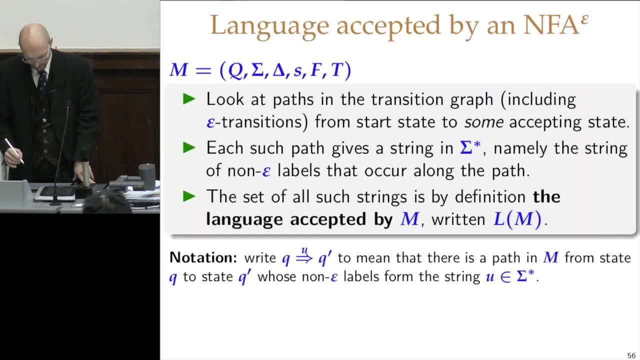 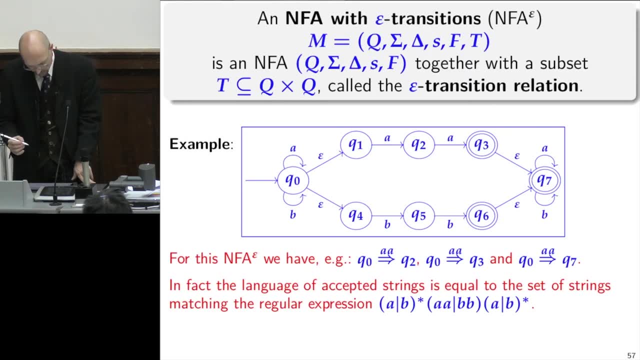 we don't have all these backslashes, backslashes now. this is what we just said in the formal definition. you take the same things as you had before for the NFA and you add another set which is a subset of the Cartesian product of the states times themselves. 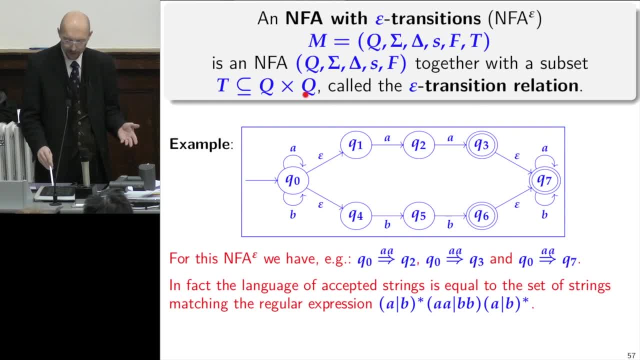 which means arrows from a state to another state that are labeled with epsilon. so this is all the arrows with an epsilon on top, from any state to any other state. if you add this relation to this tuple, you get an NFA with epsilon transitions indicated: NFA- epsilon. 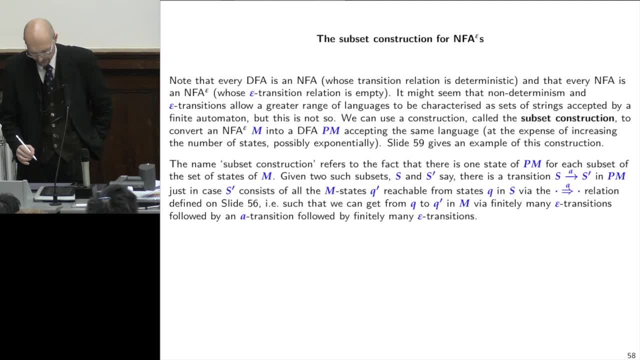 like this and you could think: okay, clearly, every deterministic finite automaton is: well, every deterministic finite automaton is also a non-deterministic finite automaton, except that the relation has this particular shape where there is a unique value for every combination of state and input symbol. 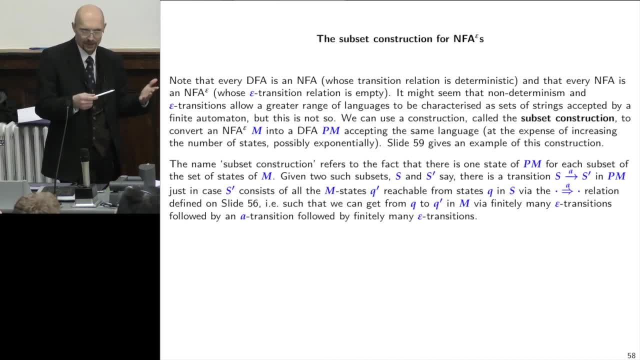 so it sounds like the NFA is a bit more than the DFA, because every DFA is also an NFA, but not vice versa. and then the NFA- epsilon. you can say: every NFA epsilon is also an NFA, so every NFA is also an NFA epsilon.